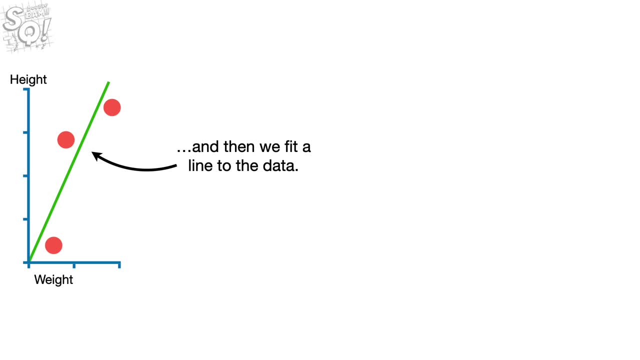 people And then we fit a line to the data. Now, if someone tells us they weigh this much, we can use the green line to predict that they are this tall Bam. Now imagine we collected height and shoe size measurements and we fit a line to the data. Now, if someone tells: 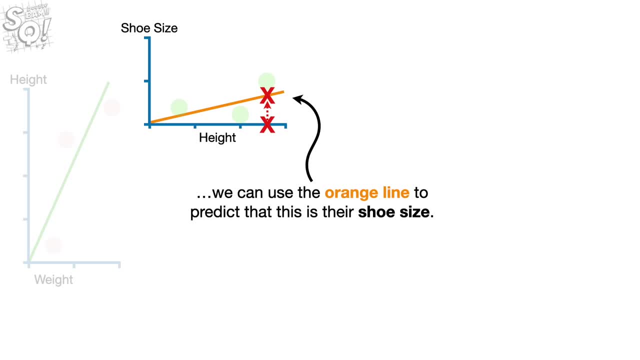 us that they are this tall, we can use the orange line to predict that this is their shoe size Bam. Now, if someone tells us that they weigh this much, then we can predict their height and we can use the predicted height to predict shoe size. And if we change the value for weight, we see a change in shoe size Bam. 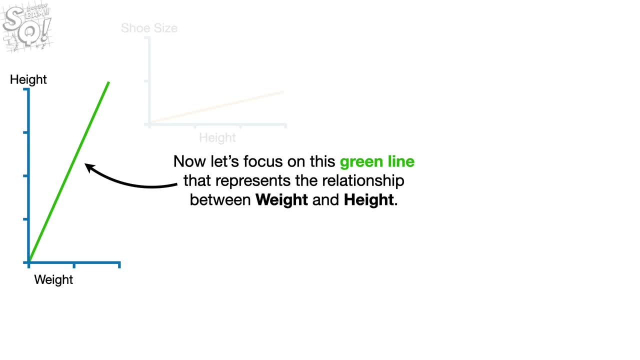 Now let's focus on this green line that represents the relationship between weight and height. We see that for every one unit increase in weight, there is a two unit increase in height. In other words, the slope of the line is 2 divided by 1, which equals 2.. And since the 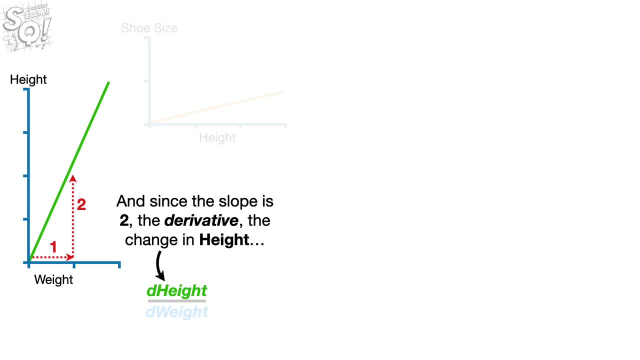 slope is two. the derivative the change in height with respect to a change in weight is two. Now, since the slope of the green line is the same as its derivative two, the equation for height is: height equals the derivative of height with respect to weight times, weight which equals 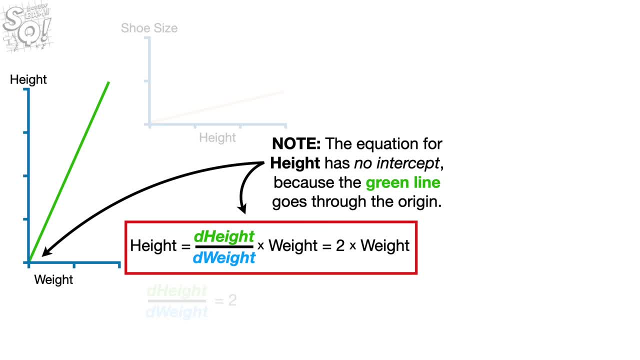 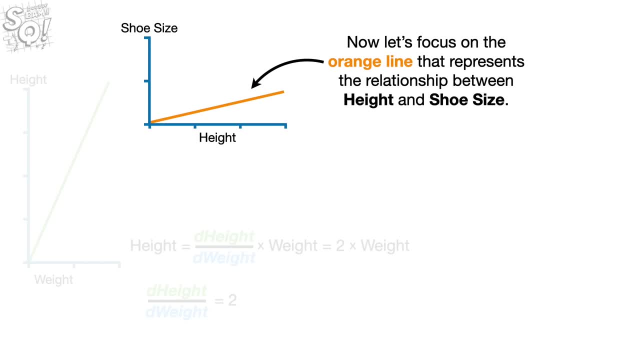 2 times weight. Note: the equation for height has no R value. Respect African brackets has no intercept because the green line goes through the origin. Now let's focus on the orange line that represents the relationship between height and shoe size. In this case, we see that for every one. 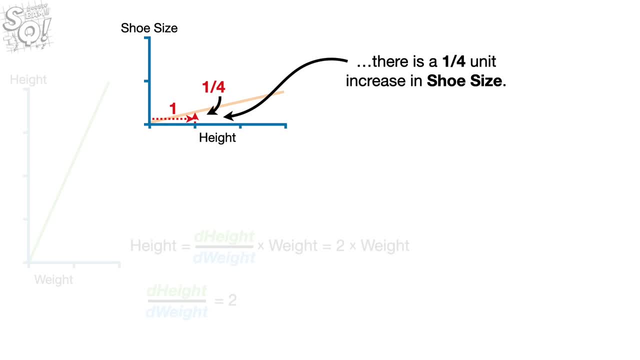 unit increase in height. there is a one quarter unit increase in shoe size, And I admit that it's hard to see the one quarter unit increase in shoe size. so just trust me, Anyway, because we go up one quarter unit for every one unit we go. 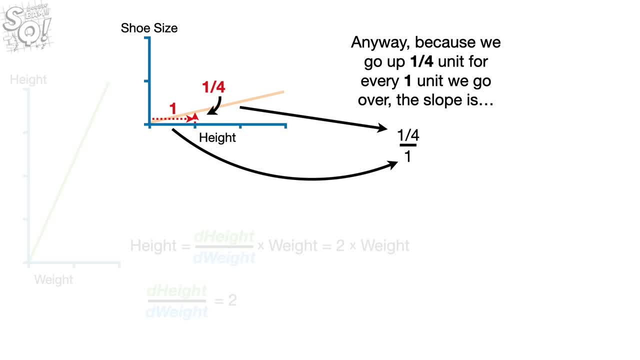 over the slope is one quarter divided by one, which equals one quarter. And since the slope is one quarter, the derivative, or the change in shoe size with respect to a change in height, is one quarter. Now, since the slope of the orange line is: 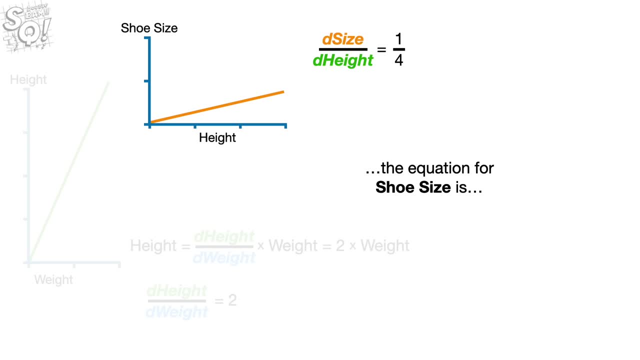 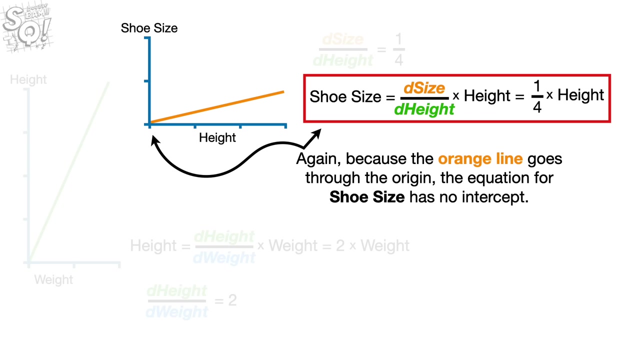 the same as its derivative. the equation for shoe size is the same. Shoe size equals the derivative of shoe size with respect to height times height, which equals one quarter times height. And again, because the orange line goes through the origin, the equation for shoe size has no 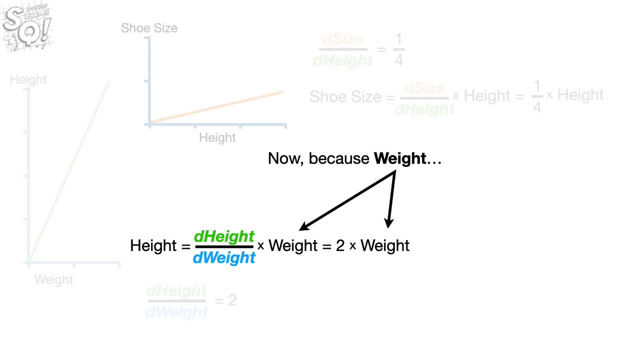 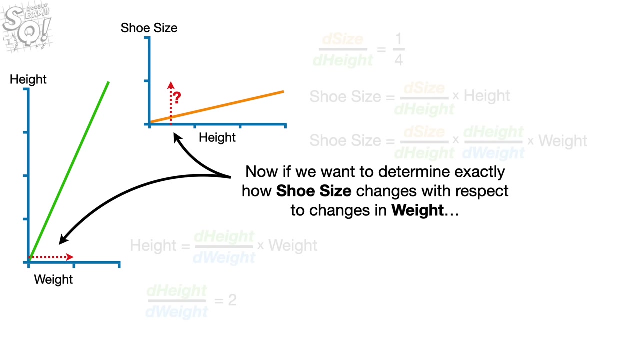 intercept. Now, because weight can predict height and height can predict shoe size, we can plug the equation for height into the equation for height, The equation for shoe size. Now, if we want to determine exactly how shoe size changes with respect to changes in weight, we can take the 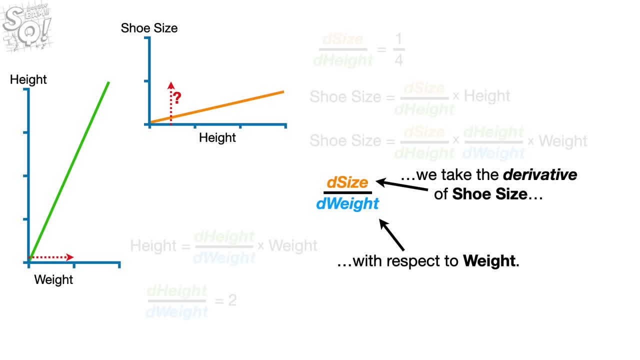 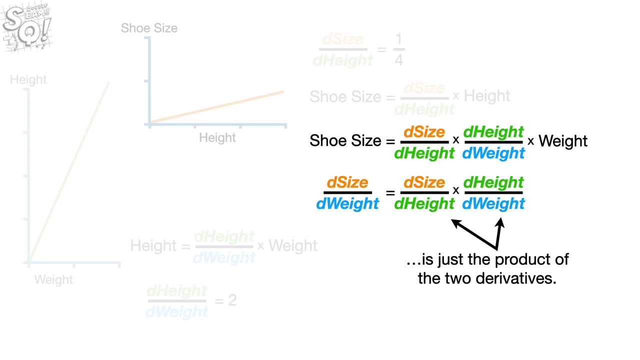 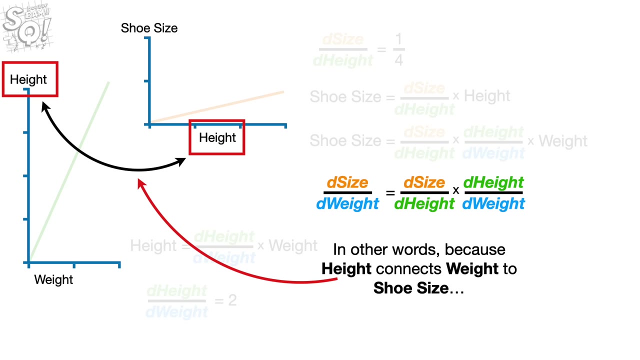 derivative of shoe size with respect to weight And the derivative of the equation for shoe size with respect to weight is just the product of the two derivatives. In other words, because height connects weight to shoe size, the derivative of shoe size with respect to weight. 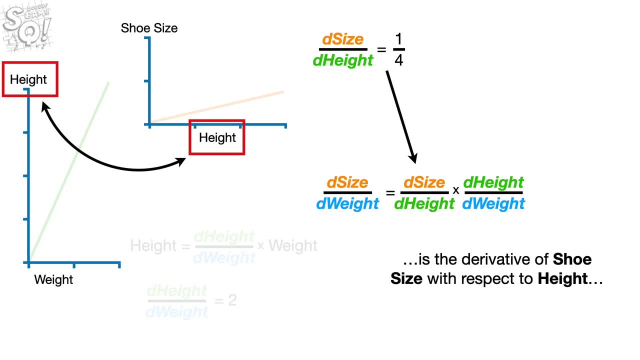 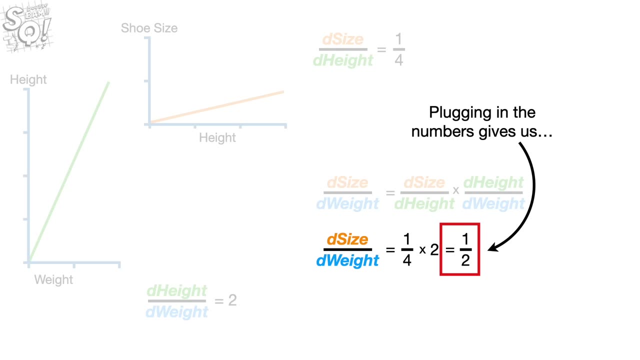 is the derivative of shoe size with respect to height, times, the derivative of height with respect to weight. This relationship is the essence of the chain rule. Plugging in numbers gives us one half, And that means for every one unit increase in weight. beep, boop, beep. 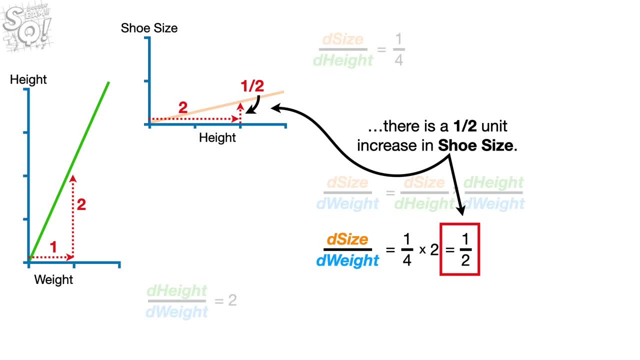 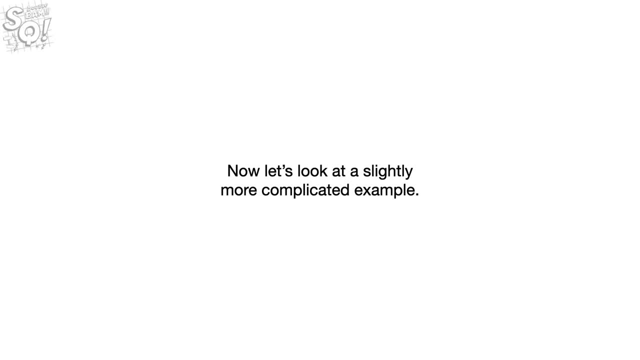 there is a one half unit increase in shoe size Bam. Now let's look at a slightly more complicated example. Imagine we measured how hungry a bunch of people were and how long it had been since they last had a snack, As time since the last snack increases on the x-axis. 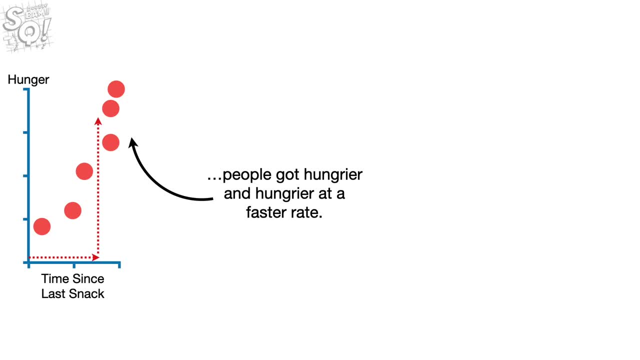 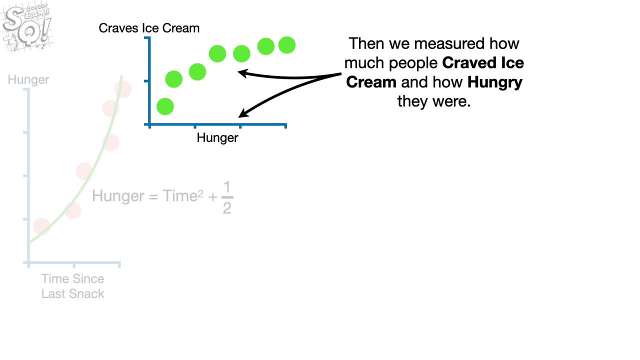 people got hungrier and hungrier at a faster rate. So we fit an exponential line with intercept one-half to the measurements to reflect the increasing rate of hunger. Then we measured how much people craved ice cream and how hungry they were. The hungrier someone was, the more they craved ice cream. 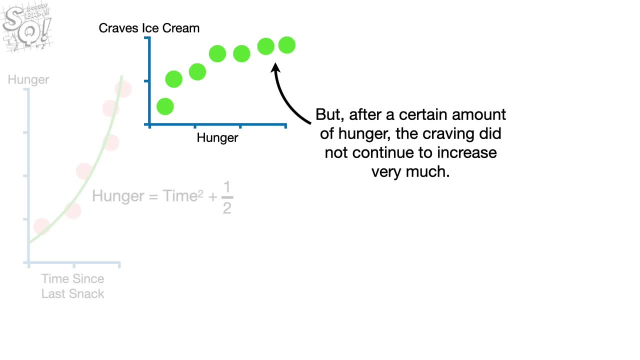 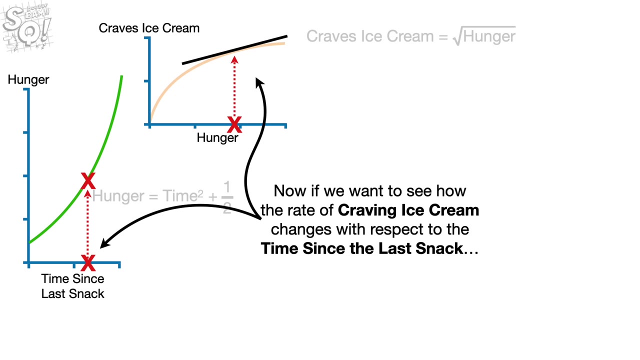 But after a certain amount of hunger the craving did not continue to increase very much. So we fit a square root function to the data to reflect how the increase in craving tapers off. Now, if we want to see how the rate of craving ice cream changes, with respect, 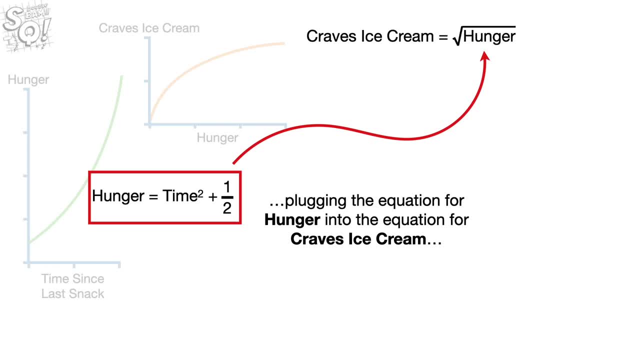 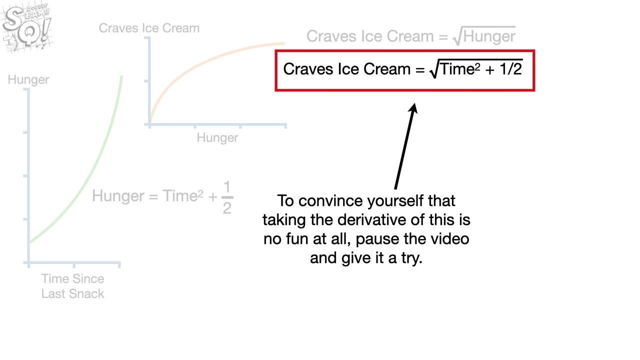 to the time since the last snack, Plugging the equation for hunger into the equation for craves, ice cream gives us an equation without an obvious derivative. To convince yourself that taking the derivative of this is no fun at all, Pause the video and give it a try. 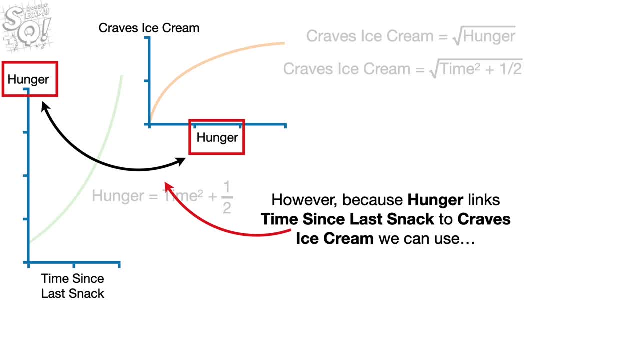 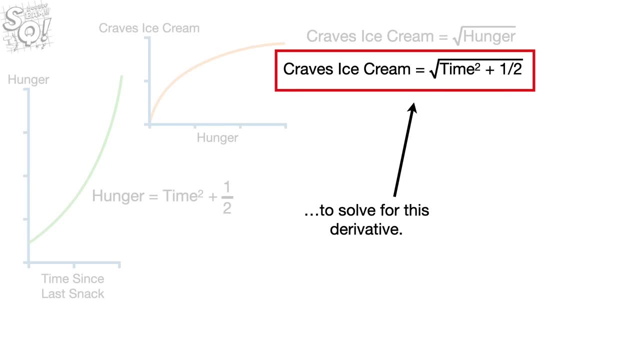 However, because hunger is a derivative of craving ice cream and hunger links time since last snack to craves ice cream, we can use the chain rule to solve for this derivative. First, the power rule tells us that the derivative of hunger with respect to the 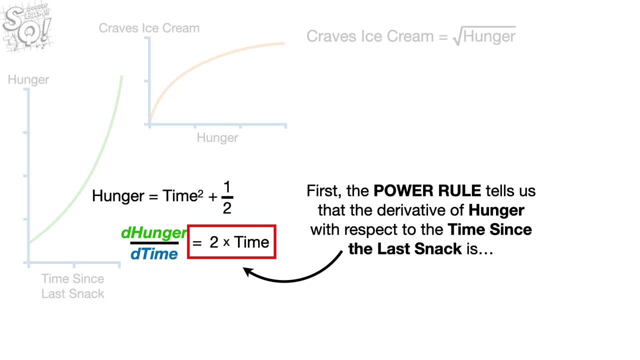 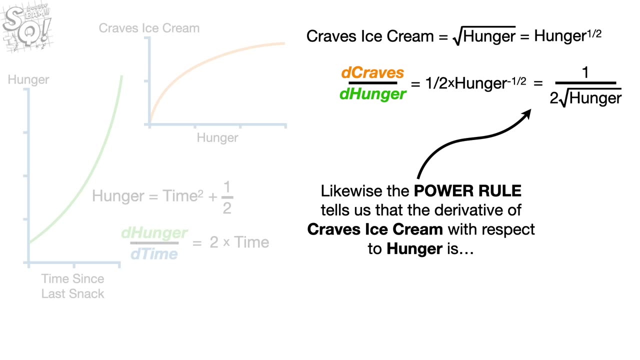 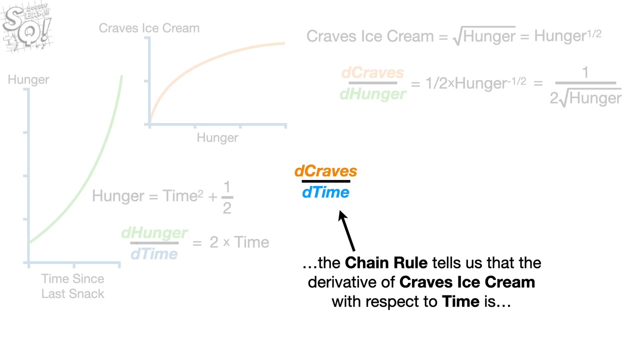 time, since the last snack is two times time. Likewise, the power rule tells us that the derivative of craves ice cream with respect to hunger is one divided by two times the square root of hunger. So, with these two derivatives, the chain rule tells us that the derivative of craves ice cream with 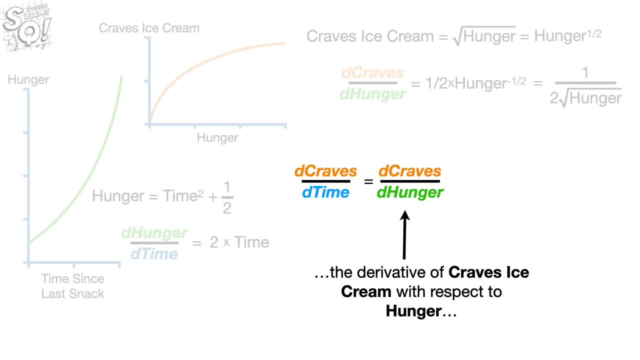 respect to time is the derivative of craves, ice cream with respect to hunger times, the derivative of hunger with respect to time since last snack. So we plug in the derivatives Beep, boop, beep And plug in the equation for hunger. 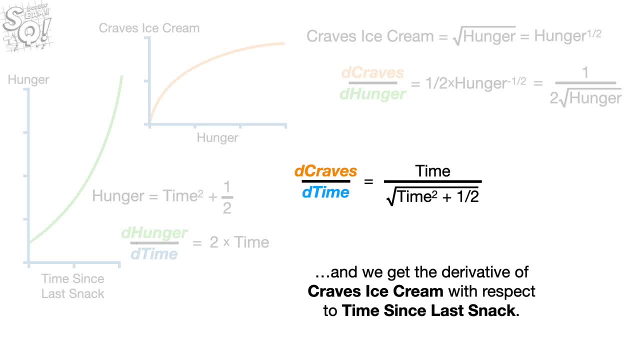 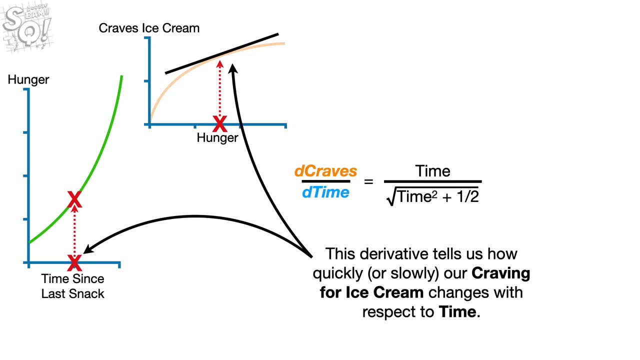 And cancel out the twos And we get the derivative of craves ice cream with respect to time since last snack. This derivative tells us how quickly or slowly our craving for ice cream changes with respect to time. Double bam In this last example. 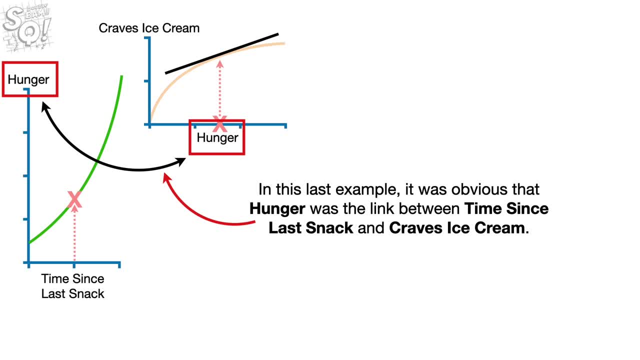 it was obvious that hunger is a derivative of craving ice cream. with respect to time, It was obvious that hunger was the link between time since last snack and craves ice cream, And we had an equation for hunger in terms of time and an equation for craves ice cream in terms of hunger. 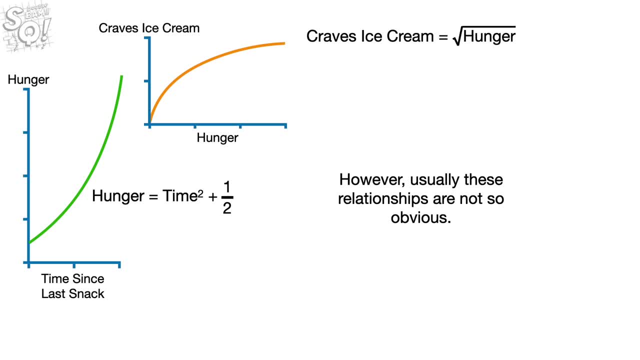 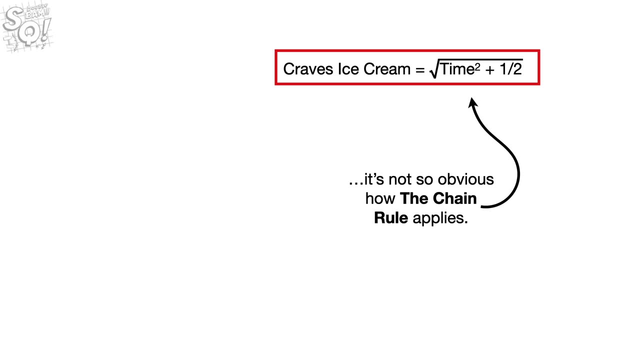 However, usually these relationships are not so obvious. Instead of having two separate equations, we usually get the first equation jammed into the second, And when all you have is this, it's not so obvious how the chain rule applies. So we can talk about how to apply the chain rule in this situation. 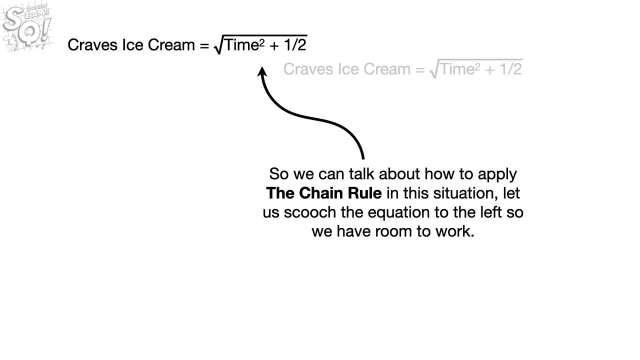 Let us scooch the equation to the left so we have room to work. Now. one thing we can do in this situation is look for things in the equation that can be put in parentheses. For example, the square root symbol can be replaced with parentheses. 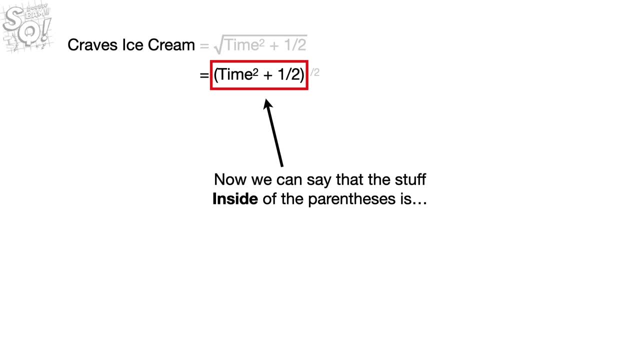 Now we can say that the stuff inside the parentheses is time squared plus one half, And craves ice cream can be rewritten as the square root of the stuff inside. Now the chain rule tells us that the derivative of craves ice cream with respect to time is: 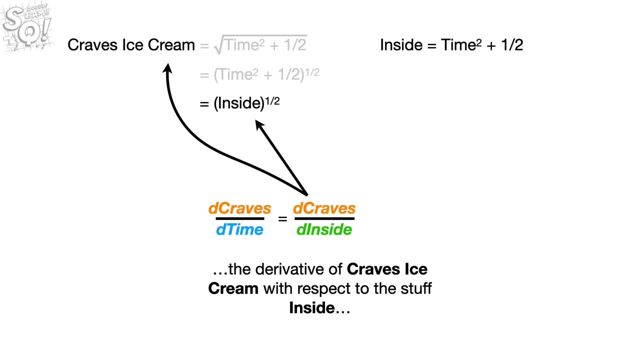 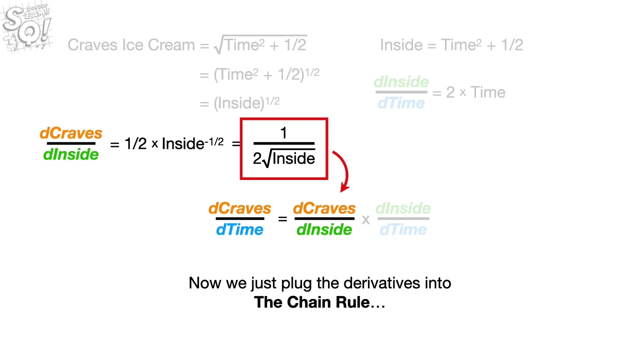 the derivative of craves ice cream with respect to the stuff inside times. the derivative of the stuff inside with respect to time. The power rule gives us the derivative of craves ice cream with respect to the stuff inside And the power rule gives us the derivative of the stuff inside with respect to time. 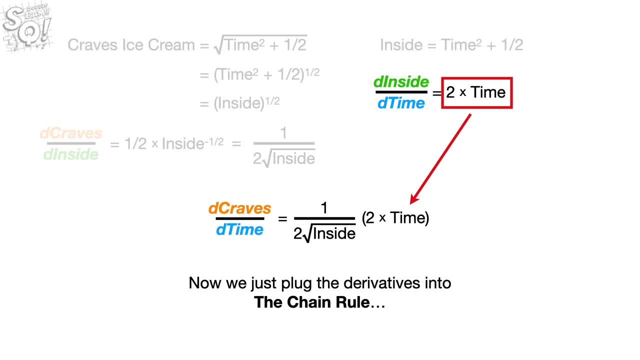 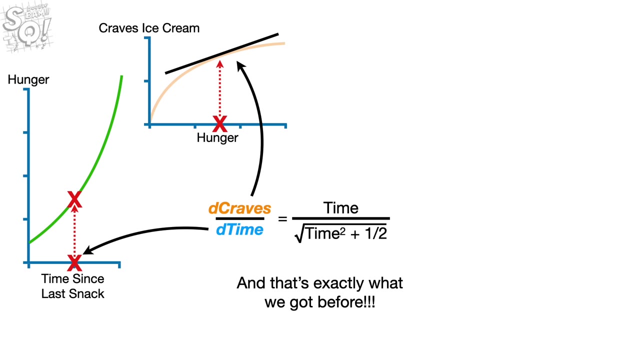 Now we just plug the derivatives into the chain rule and plug in the equation for the stuff inside. cancel out the twos and we get the derivative of craves, ice cream with respect to the time since last snack, And that's exactly what we got before. 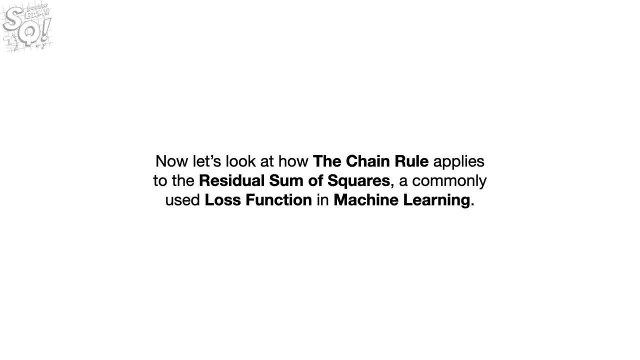 Bam. Now let's look at how the chain rule applies to the residual sum of squares, a commonly used loss function in machine learning. if this does not make any sense to you, just imagine I said: now let's look at one last example. 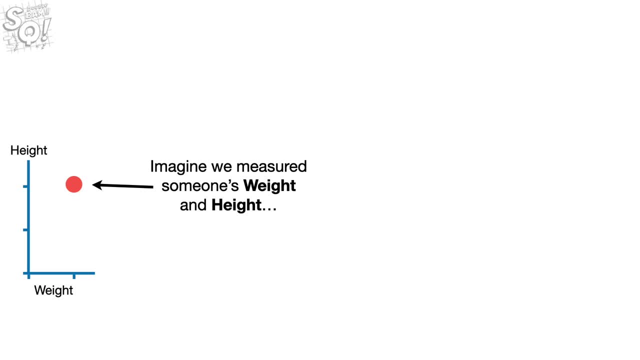 Imagine we measured someone's weight and height and we wanted to fit this green line to the measurement. Now, to keep things simple, let's assume we can only move the green line up and down. The equation for the green line is: height equals the intercept plus one times weight. 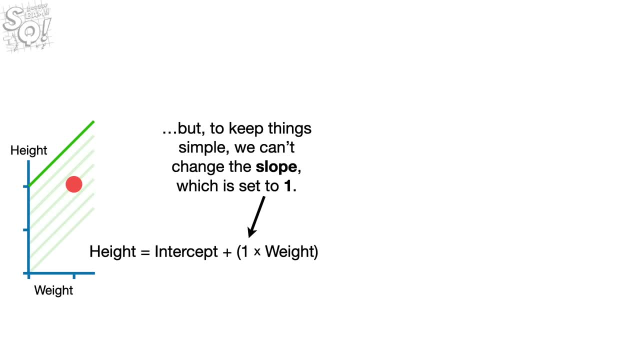 And we can change the intercept. But to keep things simple, we can't change the slope which is set to one. If we set the intercept to zero, then this location on the green line is the predicted height And we can calculate the residual. 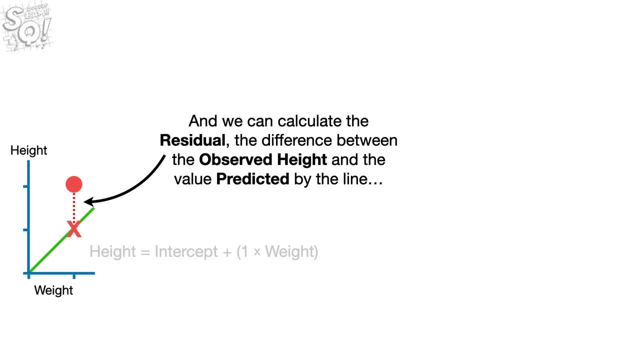 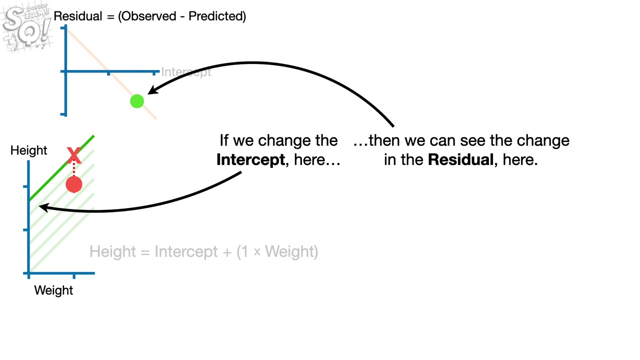 the difference between the observed height and the value predicted by the line And we can plot the residual on this graph, which has the intercept on the x-axis and the residual on the y-axis. If we change the intercept here, then we can see the change in the residual here. 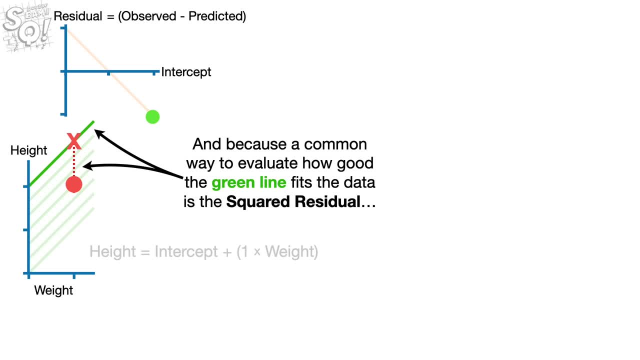 And because a common way to evaluate how good the green line fits the data is the squared residual. we can plot the squared residual here where we have the residuals on the x-axis and the squared residuals on the y-axis. Now, if we change the intercept here, 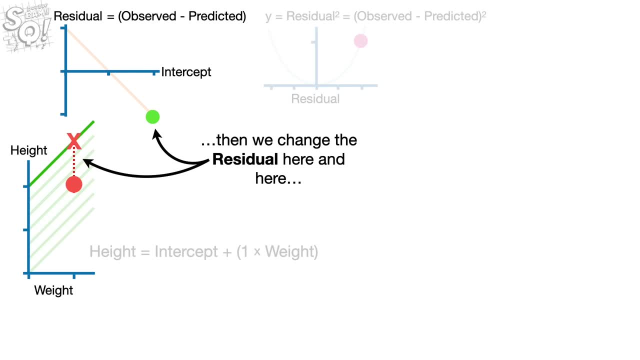 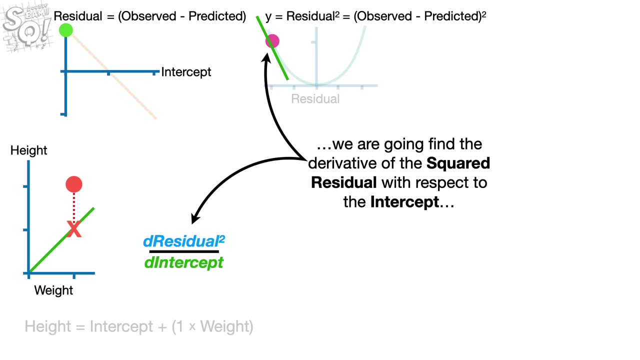 then we change the residual here and here, And changing the residual here changes the squared residual here. In order to find the value for the intercept that minimizes the squared residual, we are going to find the derivative of the squared residual with respect to the intercept. 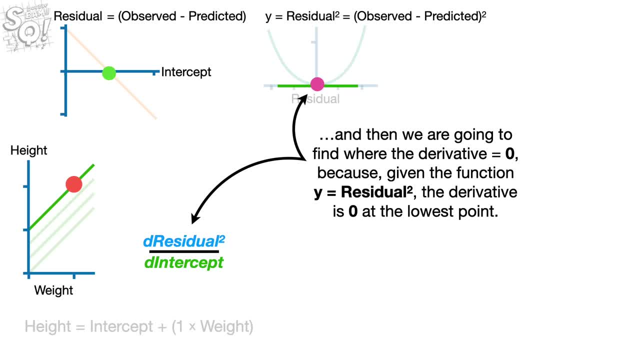 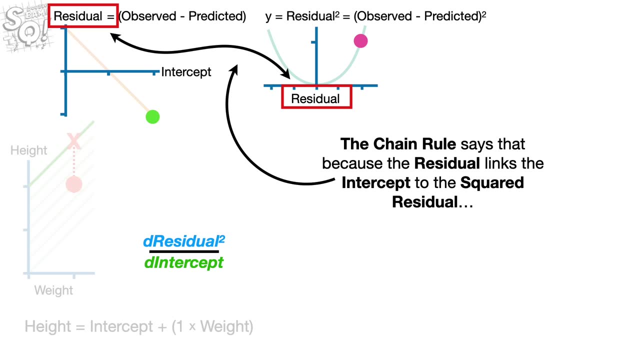 And then we're going to find where the derivative equals zero, because, given the function y equals the residual squared, the derivative is zero at the lowest point. The chain rule says that because the residual links the intercept to the squared residual, then the derivative of the squared residual 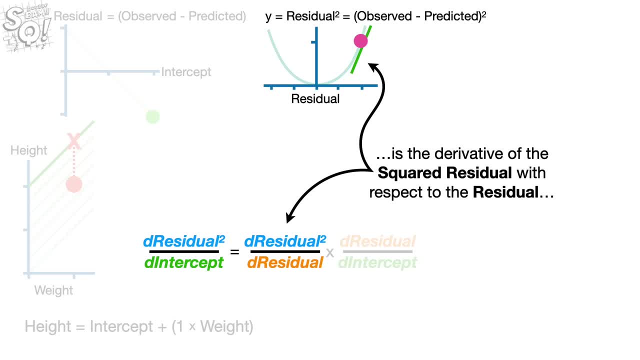 with respect to the intercept. is the derivative of the squared residual with respect to the residual times the derivative of the residual with respect to the intercept? The power rule tells us that the derivative of the residual squared is just two times the residual, So let's plug that in. 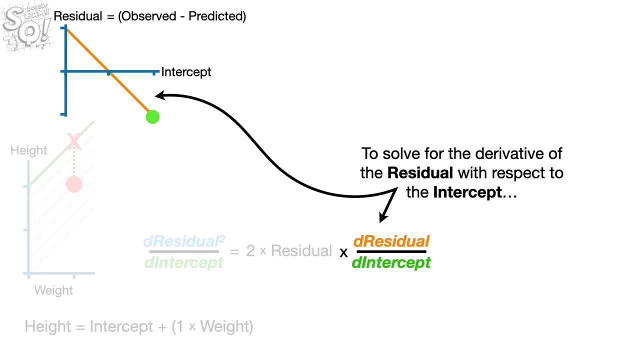 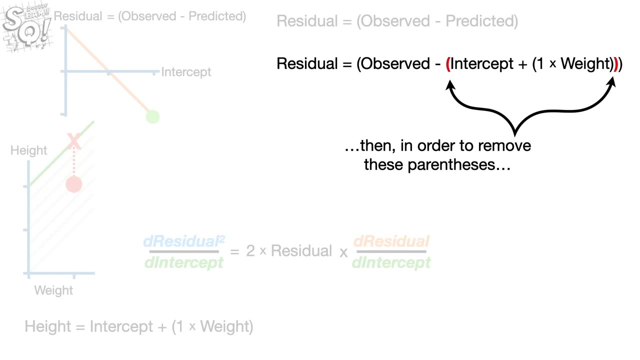 To solve for the derivative of the residual with respect to the intercept. we move the equation for the residual over here, so we have room to work. Then we plug in the equation for the predicted height. Then, in order to remove these parentheses, we multiply everything inside by negative one. 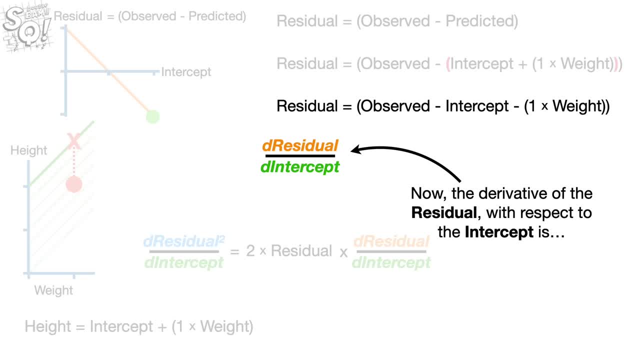 Now the derivative of the residual with respect to the intercept is zero, because this term does not contain the intercept, plus negative one. because the derivative of the negative intercept equals negative one Plus zero, because the last term does not contain the intercept. Now do the math. 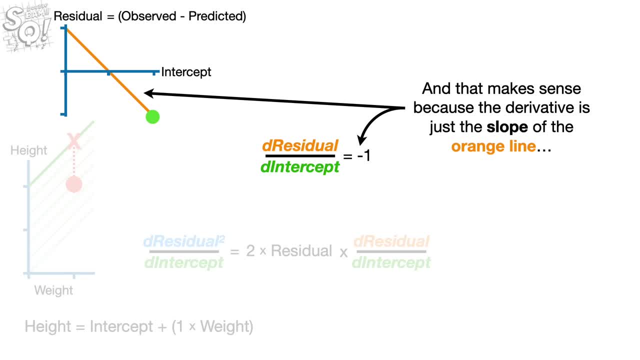 and we are left with negative one. And that makes sense, because the derivative is just the slope of the orange line, And by i we can see that the slope of the orange line is negative one. So let's plug this derivative in here and do a little math. 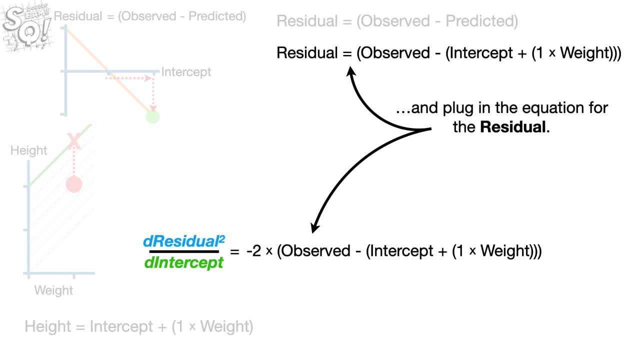 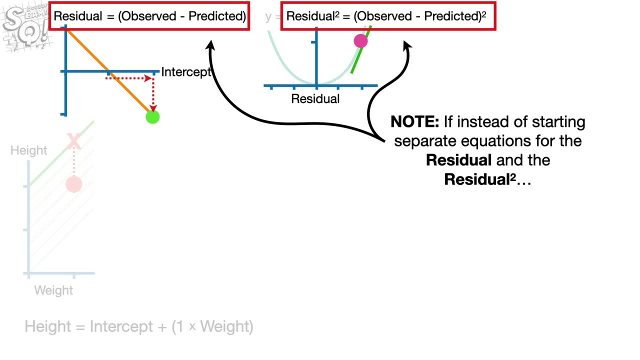 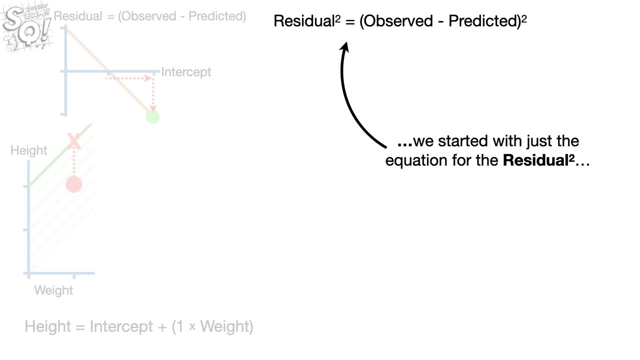 and plug in the equation for the residual. Now we have the derivative for the residual squared in terms of the intercept. Note if, instead of starting with separate equations for the residual and the residual squared, we started with just the equation for the residual squared. 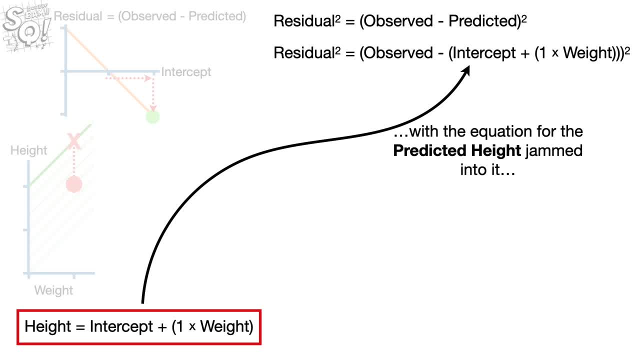 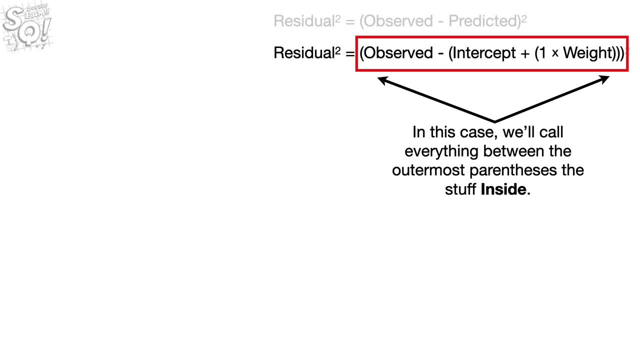 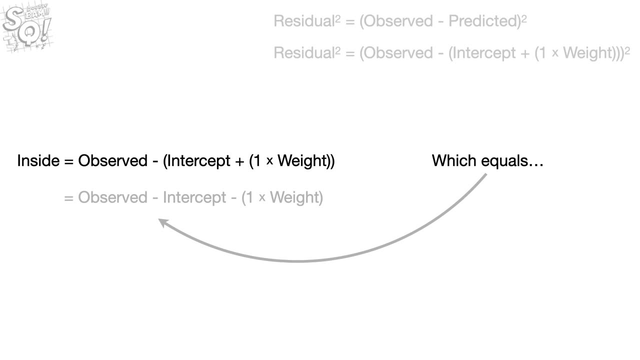 with the equation for the predicted height jammed into it. then, just like before, we can use parentheses to help us out. In this case, we'll call everything between the outermost parentheses the stuff inside, which equals the observed minus the intercept. 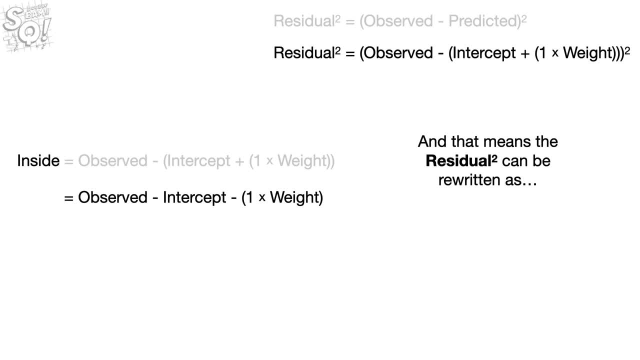 minus one times weight, And that means the residual squared can be rewritten as the square of the stuff inside. Now we can use the chain rule to determine the derivative of the residual squared. with respect to the intercept, It's the derivative of the residual squared.